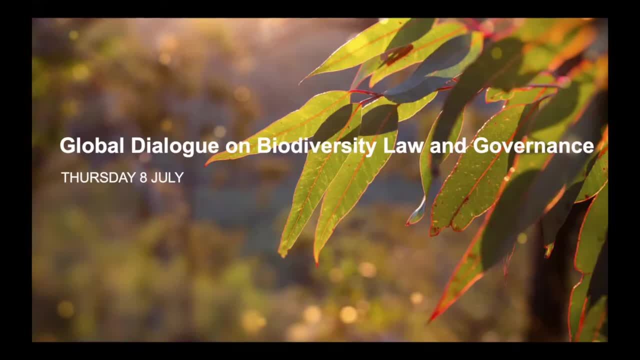 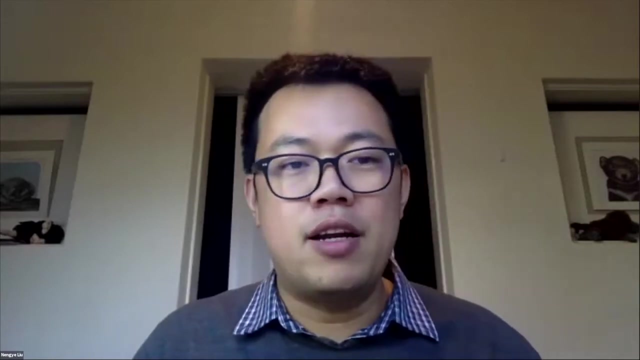 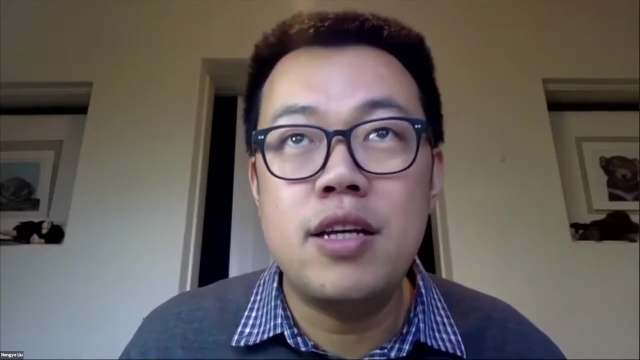 All right, good morning, good afternoon and good evening everyone. Welcome to the last day of our global dialogue on biodiversity law and governance After two. I hope you enjoyed the past two days. We did have very fruitful and inspiring discussions, And today, 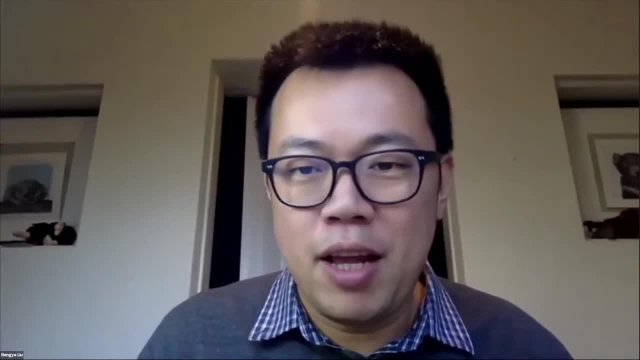 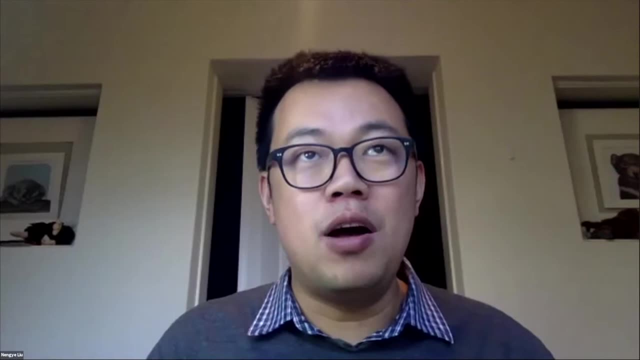 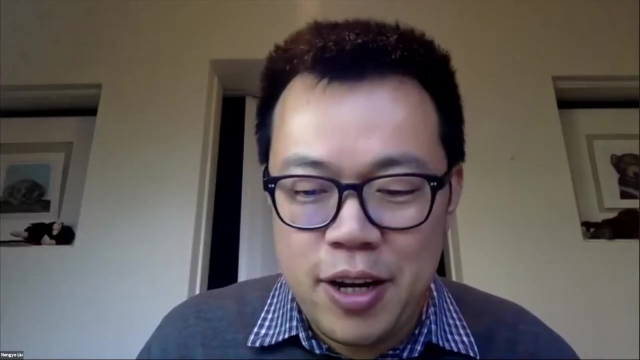 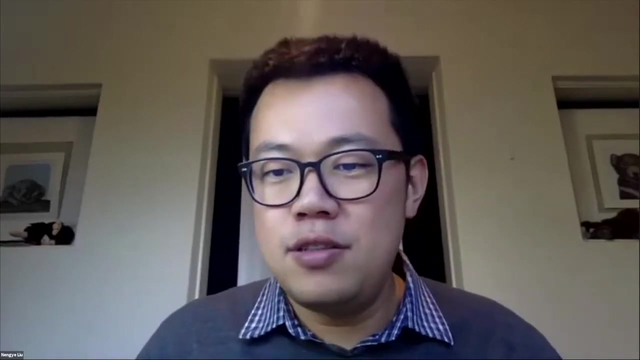 is going to be promised to be another very interesting day, And this morning we are very, very lucky to have a panel on ocean again and with speakers from the United States, Brazil, Australia and China. So, for those who just joined us for the first time, my name is Nian Liu. I'm the director. 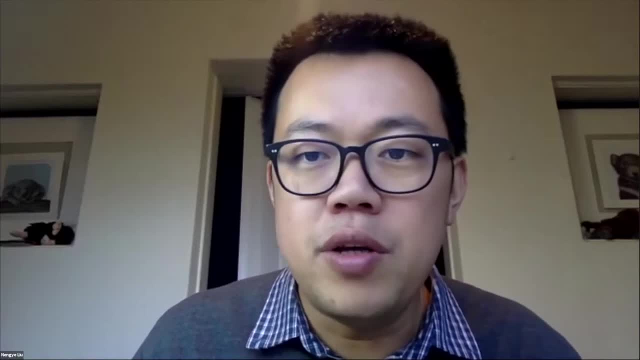 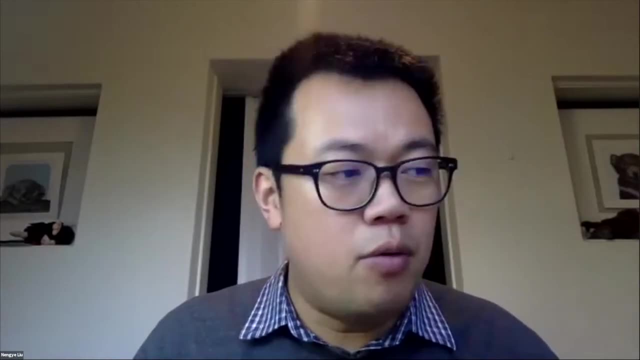 of the Center for Environmental Law here at Macquarie University, who is organizing this conference? And I won't read out our presenters' stunning profiles, which are already kind of very well elaborated in our conference booklet. So if you are interested in who, 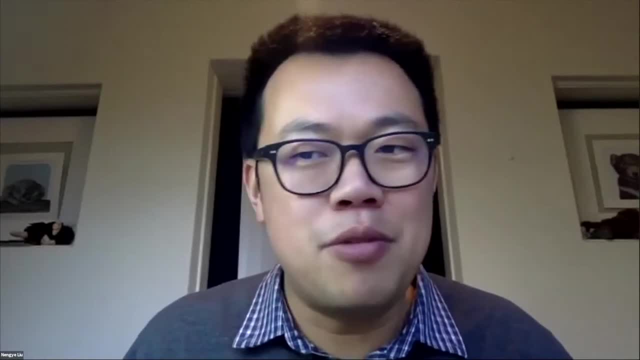 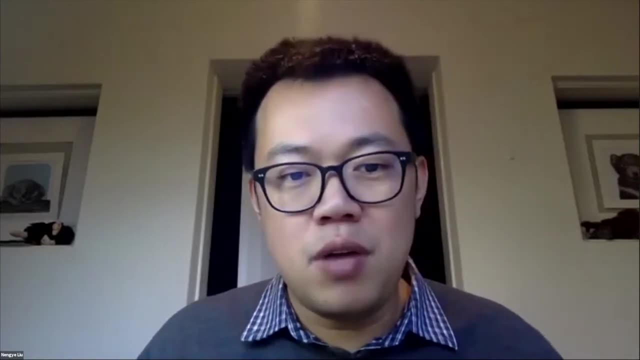 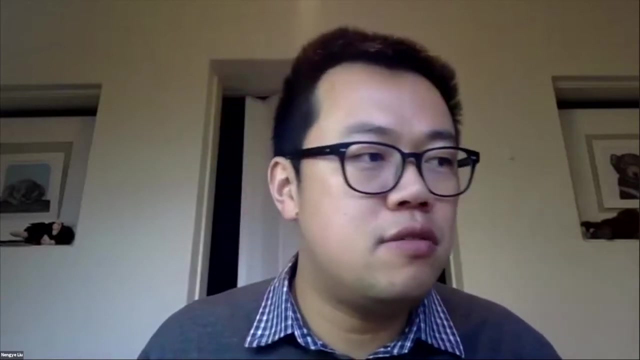 they are. I would recommend you just go through them. What we are going to do is each presentation will last around 10 to 15 minutes. While our Q&A function is open, our chat box is open, So if you have any questions, feel free to. 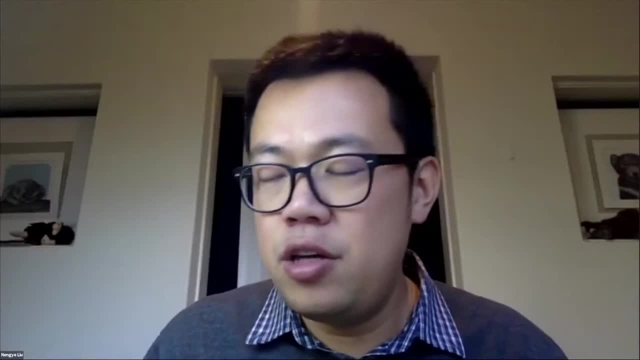 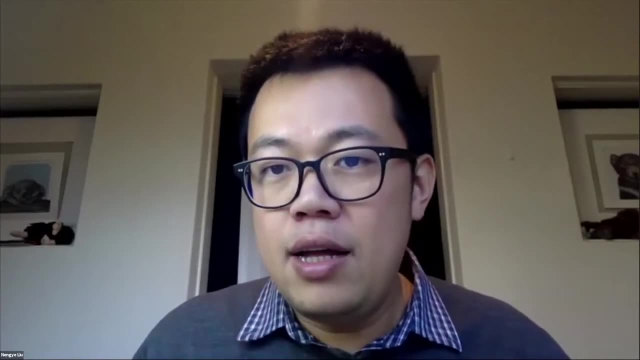 just drop your questions in either Q&A box or chat box and our panelists will answer them either by typing or live, And we will finish one presentation after another, And once we finish all the presentations, we will go to the next one. So if you have any questions, 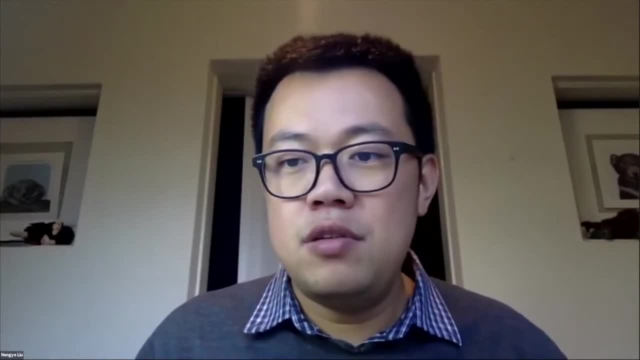 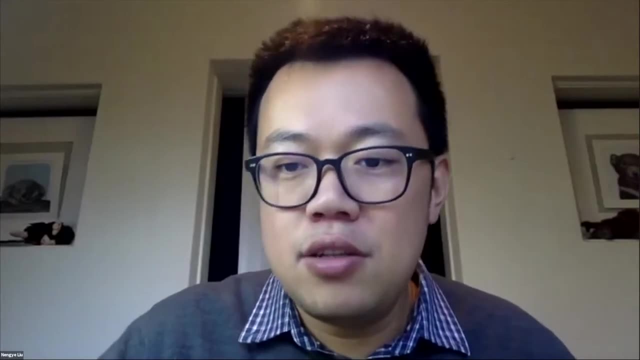 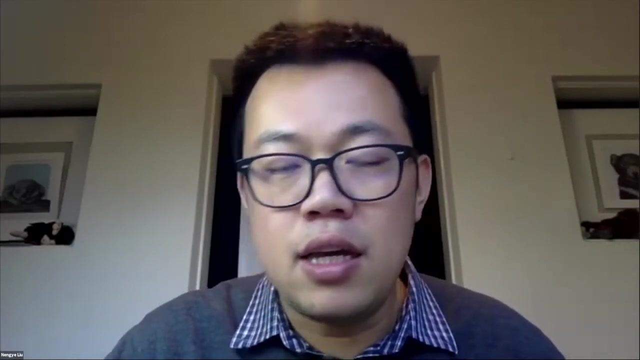 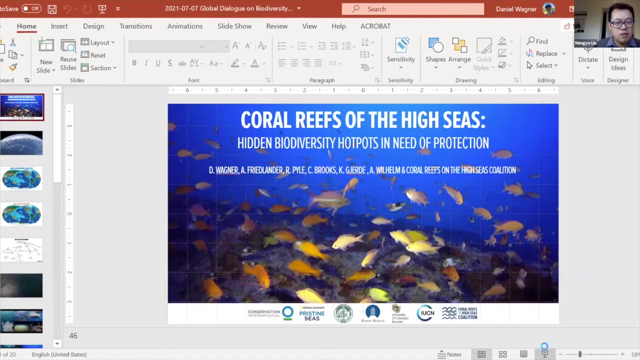 then we will start our discussions and debate. So, without further delay, it is my great pleasure to introduce Dr Daniel Wagner. Daniel is an ocean science advisor at Conservation International who is based in Washington DC, United States, I believe. So Daniel's topic is about coral reefs- coral reefs of the high seas hidden. 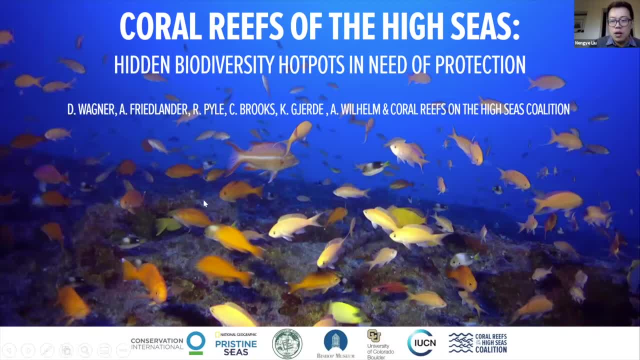 biodiversity hotspots in need of protection. Daniel Wagner, Associate Professor, Conservation International, Washington DC. So Daniel's topic is about coral reefs- coral reefs of the high seas- hidden biodiversity hotspots in need of protection. So the floor is yours. 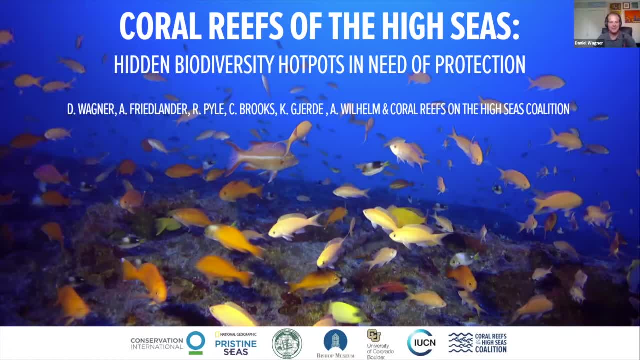 Dr Daniel Wagner, Associate Professor, Conservation International, Washington DC. Wonderful, Thanks so much. And yeah, good morning, good afternoon, good evening everyone. Today I'm going to be presenting work that was developed in collaboration with a BRIC group that were: 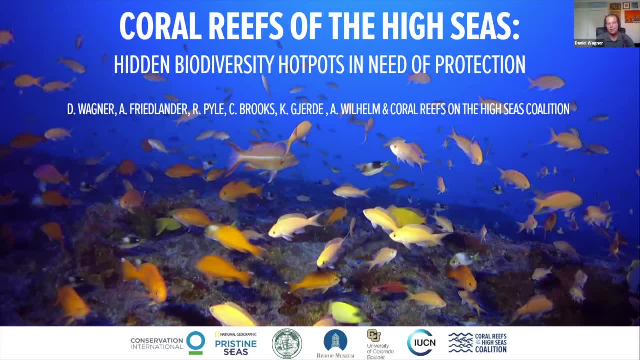 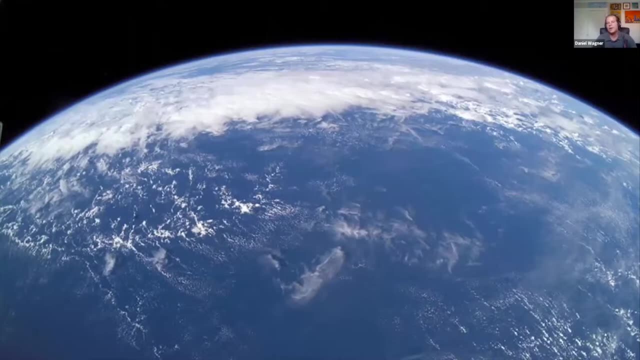 known as the Coral Reef of the High Seas Coalition. This is a big group of scientists, policy advocates, lawyers and communicators that tries to identify some most important places for protection of the high seas. So I think there's a pretty well awareness within the general population that we live. 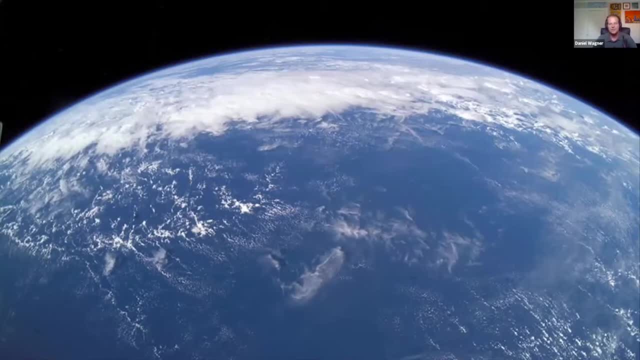 on a largely ocean planet. so 71% of the surface of our planet is covered by the ocean. But with the exception of small circles like this one and conferences and academic circles, most people don't realize that the biggest part of our ocean are areas beyond national. 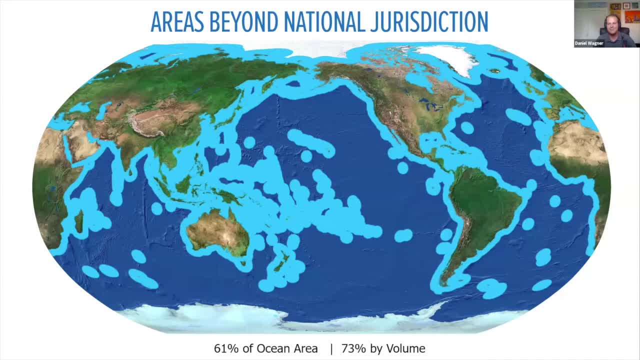 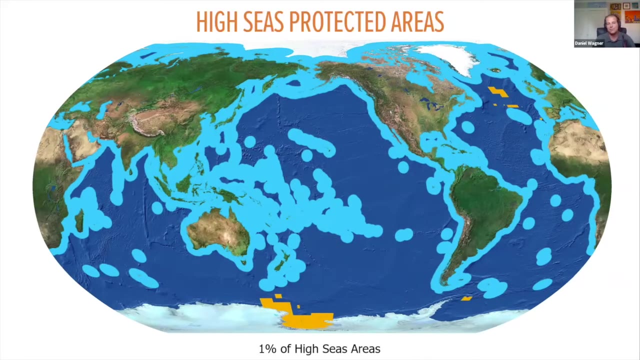 jurisdiction, this wild west where, for both law governments and biodiversity research, that covers 61% of our ocean area and 73 by volume. And what's even more alarming is that we have a very small coverage currently of conservation measures on the high seas. 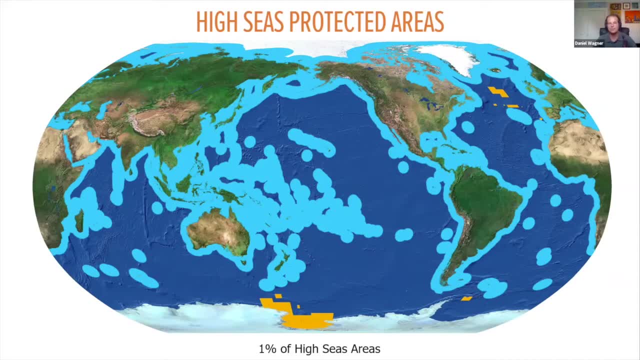 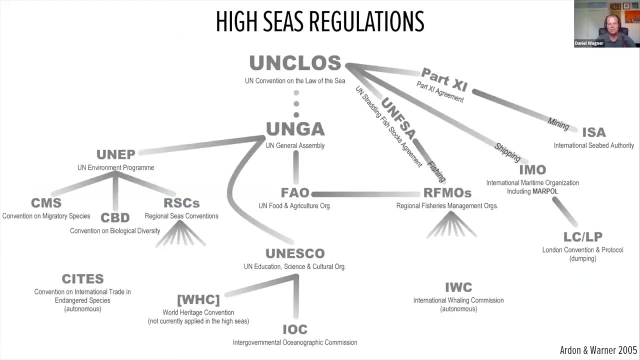 Only 1% of this vast area is currently in protection measures, And the reason for this big disparity of conservation on the high seas has to do a little bit with the complexity of how these remote ocean areas are managed. So we'll probably hear it by many of the other presenters today. a bit of the background. 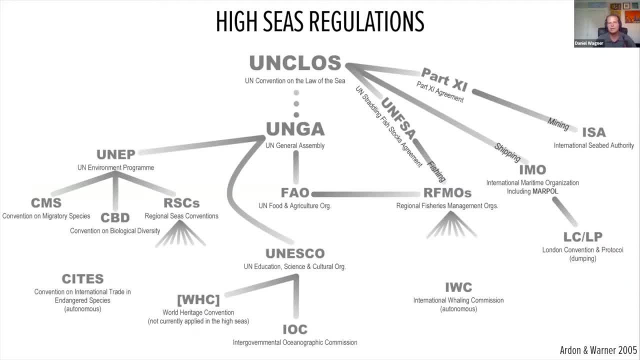 of the framework of how human activities are regulated on the high seas. So the United Nations Convention of the Law of the Sea sets the basic framework of how human uses are to be managed across the entire ocean, including in areas beyond national jurisdiction. But for areas beyond national jurisdiction it gives certain bodies the mandate to regulate. 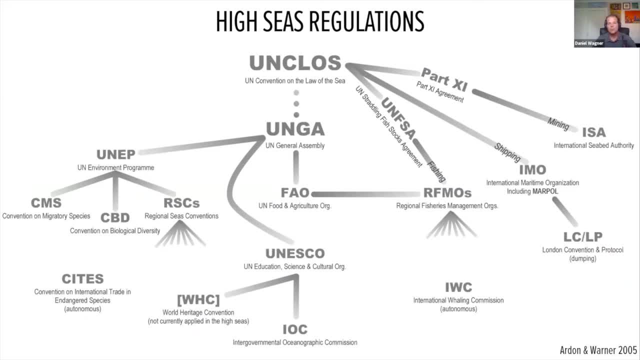 certain human activities like fishing, shipping or mining, And each one of these bodies has some kind of method for conservation. However, these are not comprehensive. There's many gaps And this makes this very challenging. So if you wanted to protect one particular, 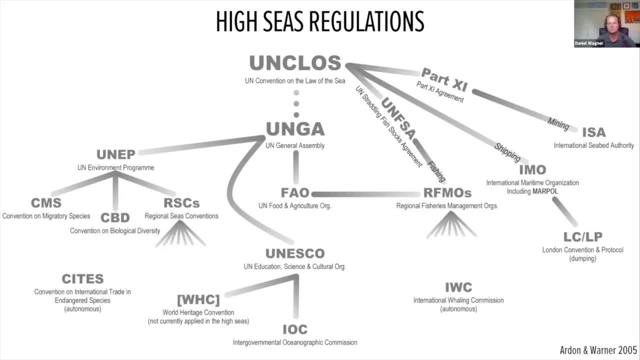 area on the high seas, you would have to go through several of these mechanisms to protect that holistically. Now, hopefully, some of this tangled mess will be untangled And I think there's a lot of evidence that's going to be necessary to protect these areas beyond. 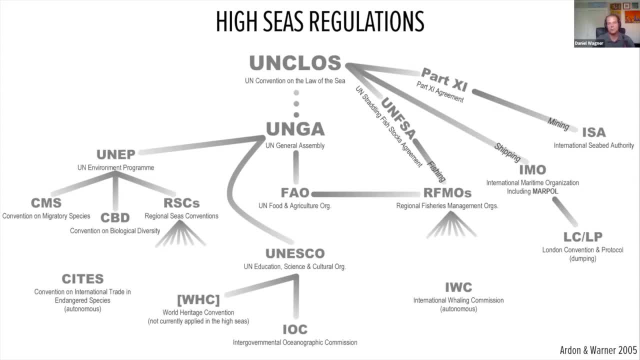 national jurisdiction. A lot of these mechanisms have been tangled in the coming years, with the high seas treated as currently under negotiation, But in the meantime, this is what we have to conserve areas beyond national jurisdiction. However, there's a bit more, even fundamental. 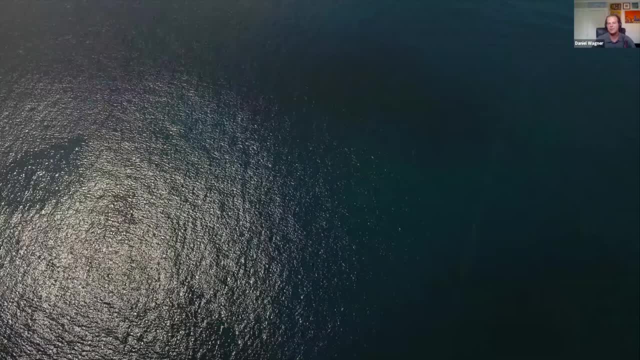 reason of why so few of the high seas are currently protected, And that really has to do with the lack of awareness that there's important places on the high seas. So for most people, when you think about the high seas, an image like the 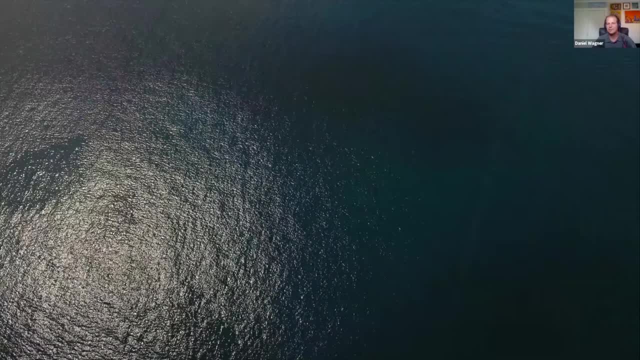 like this is all that would come to mind, something that you would look out of your airplane window when you're flying from San Francisco to Tokyo. It's this dark soup, homogenous, lifeless, where there's not much excitement. And now for people like myself and others. 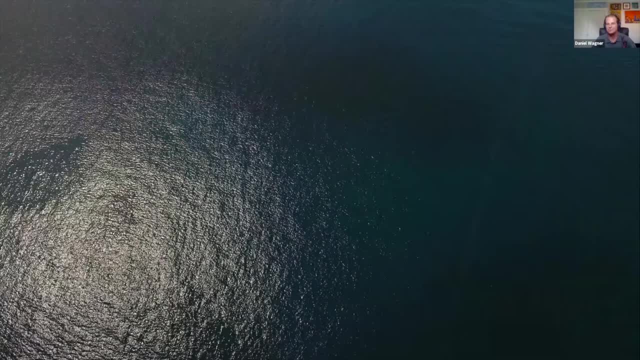 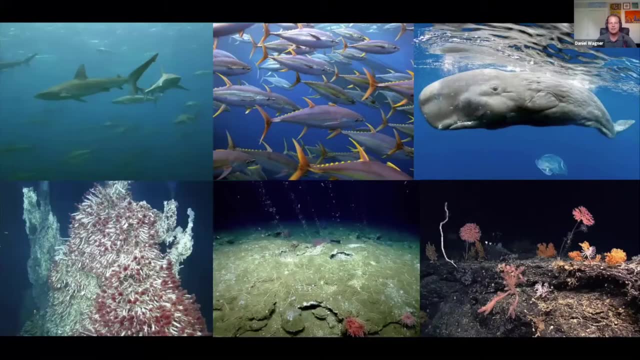 that have had the privilege to go to these remote ocean areas and actually put a submersible down and look at what's below the surface. there's some really remarkable ecosystems, anything from really diverse and productive pelagic ecosystems where you have high agglomerations of apex predators. 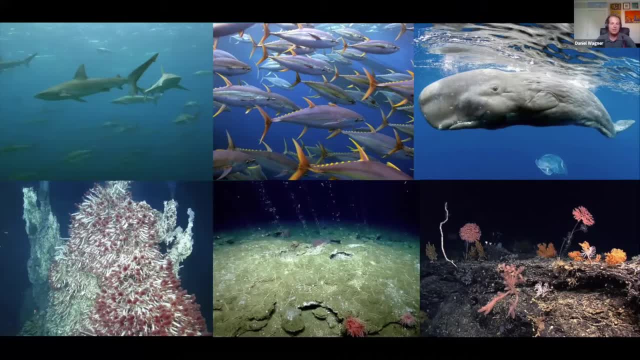 like sharks or tunas or whales, And even on the sea floor you have some pretty spectacular ecosystems, things like hydrothermal vents, things like cold water seeps, where methane and other gases come from the sea floor and fuel some pretty remarkable communities. 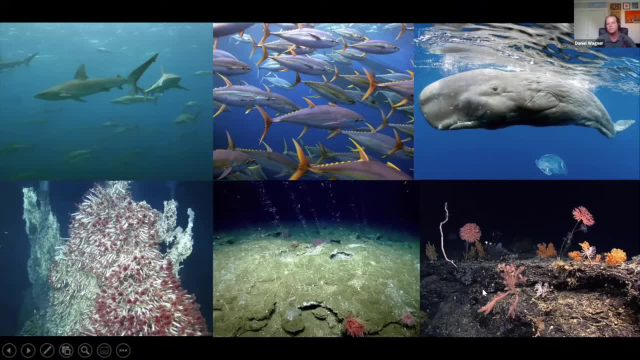 And then you also have some pretty dense communities of things like sponges and corals and others that create life for other ecosystems. Now, the problem with many of these ecosystems, while they're very productive, very diverse- these to the general population. 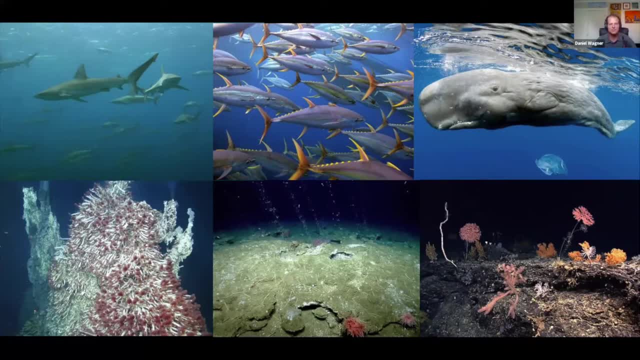 unless you happen to be an enthusiast watching the BBC or nature specials. these are things that many people don't relate to. They've never seen something like that, They will never get to see it, And since it's really difficult to to get people to care about these places, 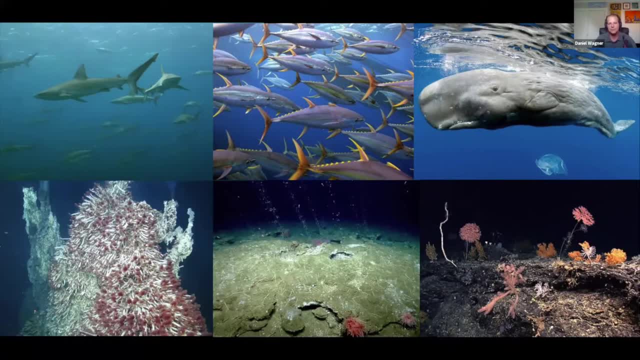 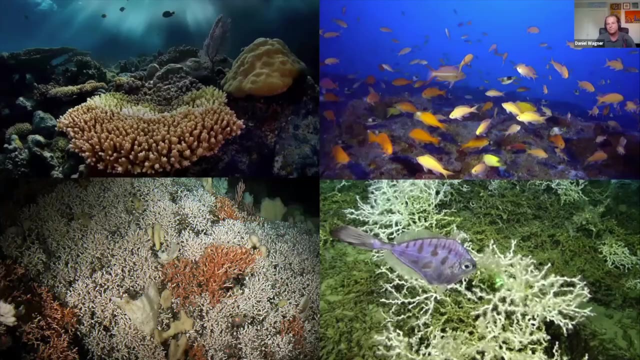 and so, as a starting point, it is important to look for things that people can relate to, to start getting awareness about conservation, And one of the ecosystems that has a long standing history of conservation in the ocean are coral reefs, And coral reefs have some of the longest lasting 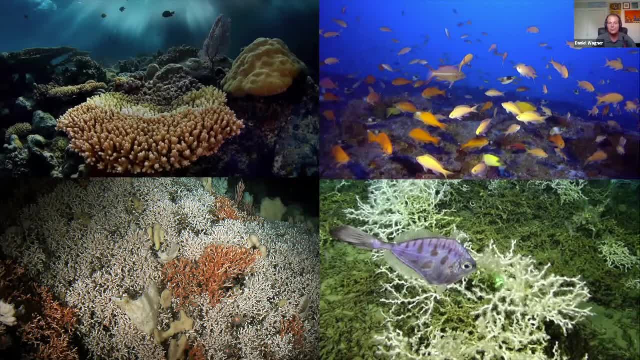 marine protected areas have been established around coral coral reefs, and this is for good reasons. Coral reefs are some of the most diverse ecosystems on the planet. About 25 percent of all species on the ocean are known to be found on coral reefs. 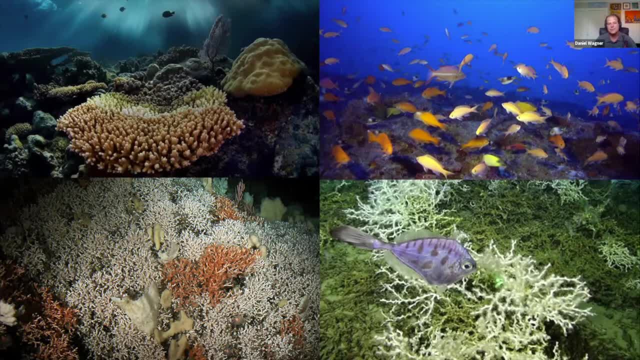 and so we have a long history of protecting them. And when I say coral reefs, these can be found across many different depths. so in shallow waters these are fueled by sunlight, but in deeper waters there's a similar species that are also found to form coral reefs. The two pictures there on the 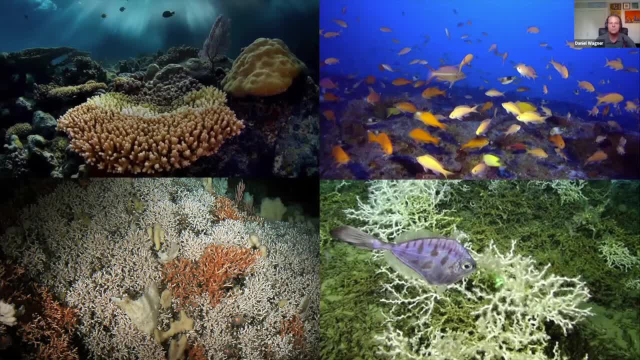 bottom. these are coral reefs that can be found at a thousand to two thousand meters, and they are also equally as diverse and productive, and so for conservation, these, these deeper cold water reefs, are just as important, and just as important to protect. So we've been 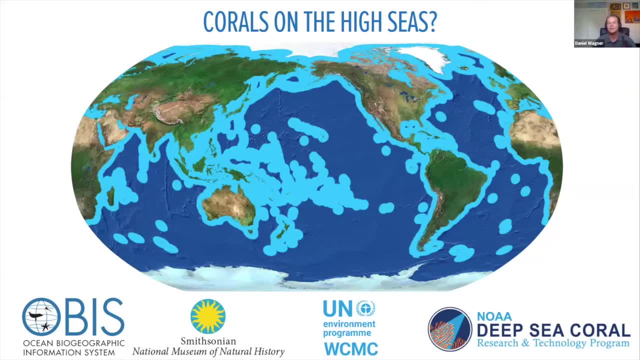 trying to answer these questions. Are coral reefs found on the high seas? This is results from a study published last year where we basically interrogated a whole bunch of publicly available databases, So these repositories of data that you can just log online and look for. 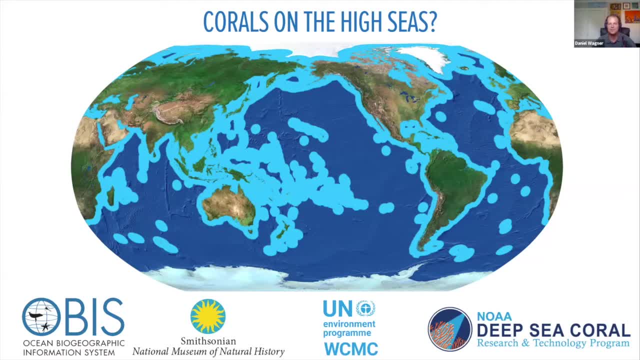 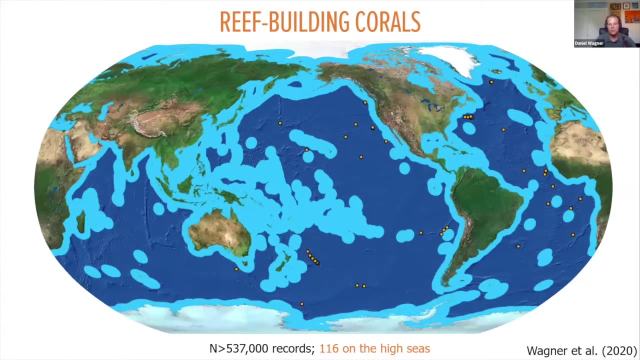 whatever your favorite animal may be and search for it and then look for where that animal is found. So these are some of the most data-rich repositories, And so just answered that very simple questions. are coral reefs found on the high seas? And lo and behold, there are quite a. 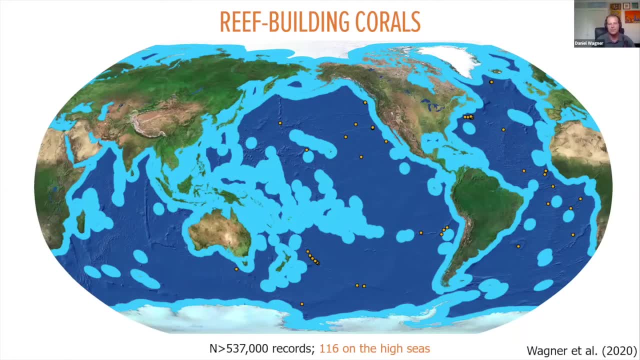 few places where we have coral reefs- about 100 or so data points confirmed coral reef locations on the high seas. And then one important point to mention here is that those 116, that's really just the tip of the iceberg, because each one of those data repositories, if you look at all the 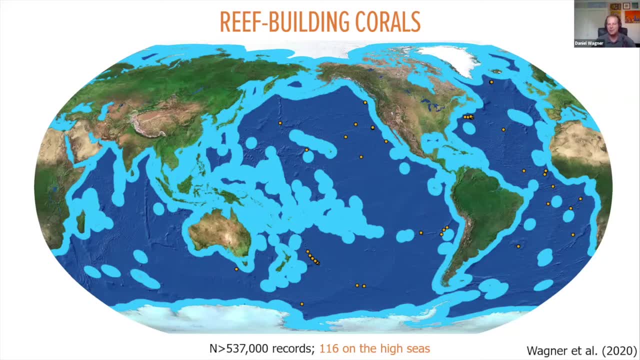 data points in it. very few of them are actually in areas beyond Africa. These places are poorly studied, poorly explored, And so the fact that we can find some data on them suggests that there's quite a bit more about them. A few more points. things about these is: 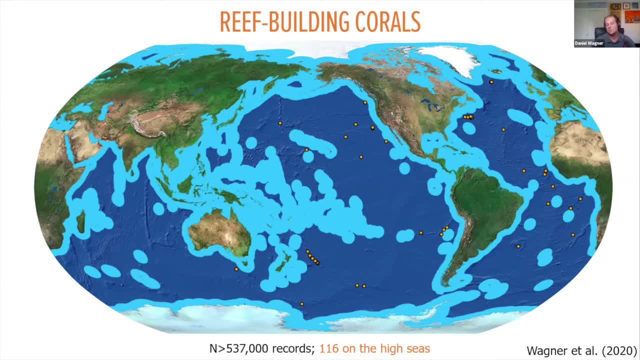 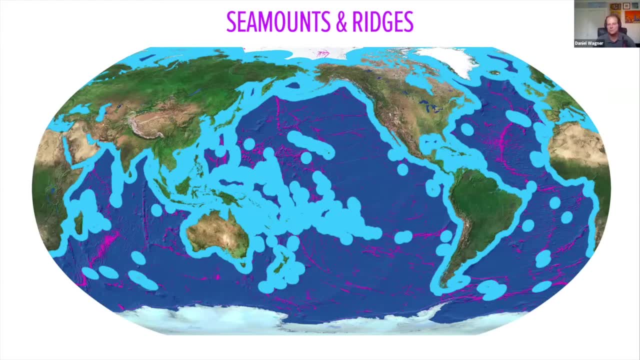 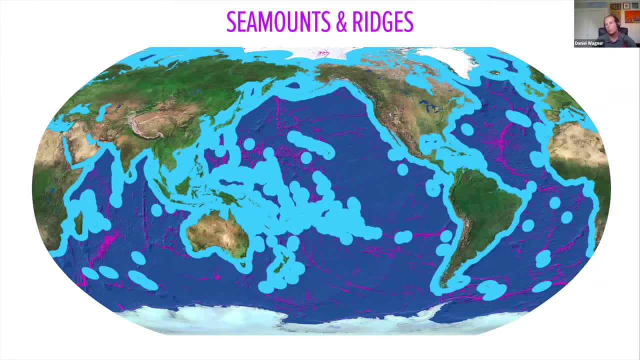 And so I just wanted to finish just by focusing on one area where we currently are focusing a lot of our efforts, and that's this area here off the coast of South America that basically connects Easter Island, or Rapa Nui, to the Peruvian coast. This is an area that is really extraordinary on. 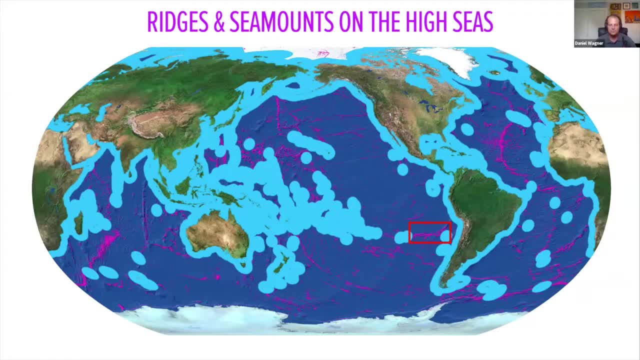 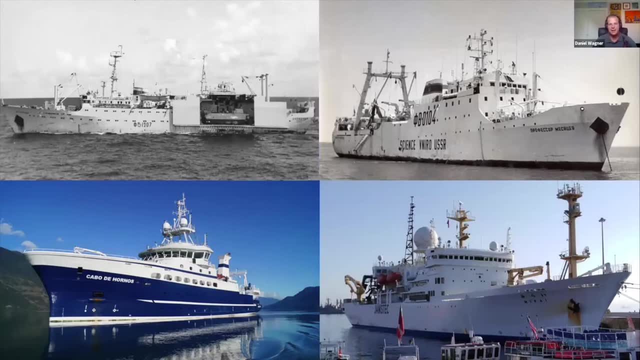 the high seas and this really should be one of its first priorities for protection on the high seas. Now, I mentioned that for most of the high seas, this is a very data poor region, So we have very limited explorations for this area. 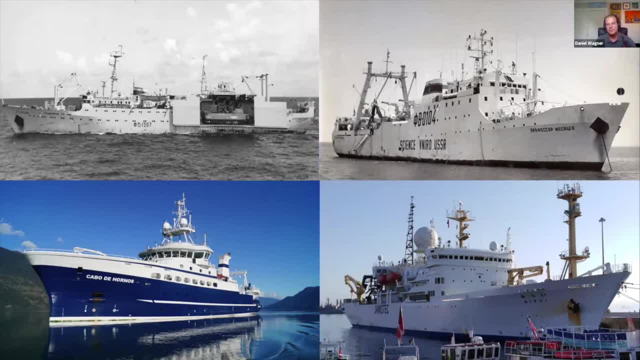 Fortunately we have quite a bit of data, and that has to do with historical explorations to this area. So there's a series of Soviet expeditions that surveyed this area in the 70s and 80s, Some more recent expeditions by Chilean. 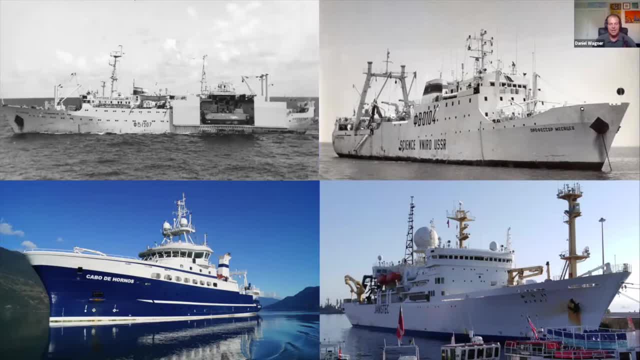 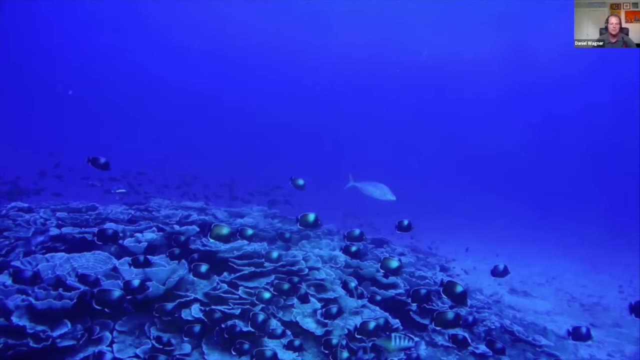 and Japanese expeditions And as a result, we have quite a bit of data, So a rich repository of- and if we dig through that data, we find some really remarkable things. So not only is this area full of coral reefs, but it's also full of other really extraordinary fauna. 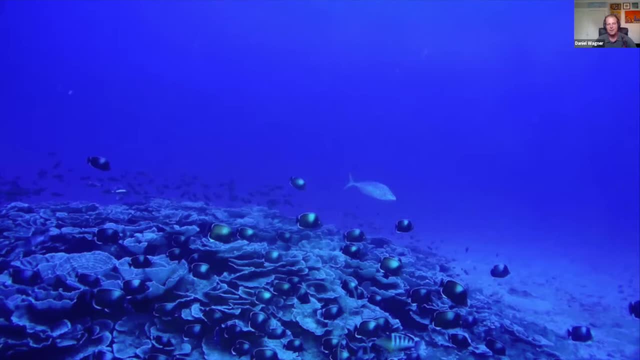 This is one of my favorite pictures of this region. And it's my favorite picture because every single animal in that picture. so you'll see all those, all those fishes, all those corals. If you would look even further, you'll see some of these elongate things. 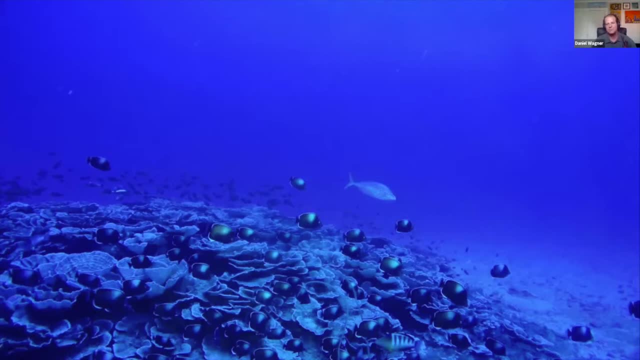 Every single animal in this picture is endemic to this region, So it means that it's only found in this region and no region else on the planet, And that makes this area really important for conservation, because if we lose these species, they're essentially extinct from our planet. 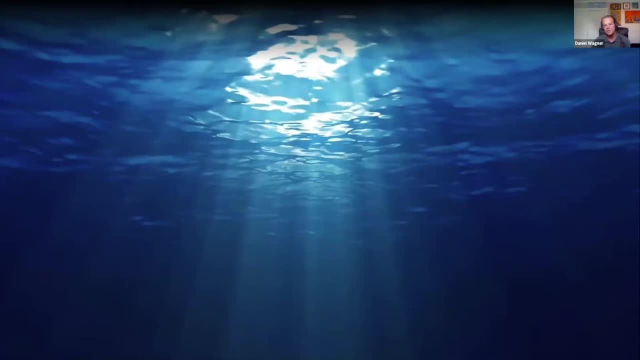 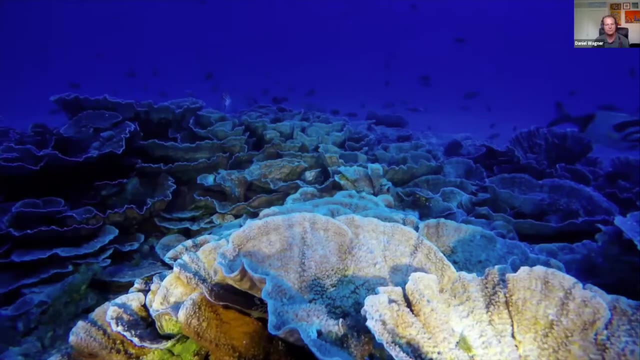 This area is also important because we have some of the clearest waters in the world here. As a result, sun can penetrate deeper and we have some of the deepest light dependent coral reefs of the world. This area is also important for vulnerable and threatened species. 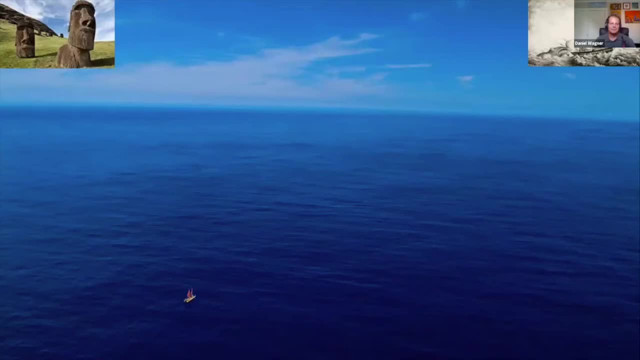 over a hundred found there. And, last but not least, this area, beyond just being important for natural significance, this area is also important for cultural significance. So I mentioned Easter Island or Rapa Nui. So there's a long history of seafaring. 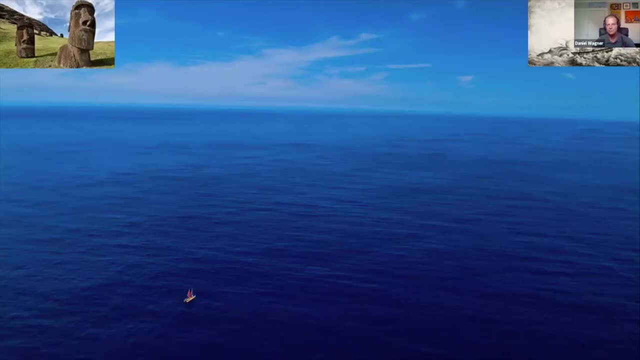 and navigation to this area. So traditional Polynesian voyages knew about this area, navigated across it, fished in these remote ocean areas. We have also some more recent whaling and other offshore activities And as a result, we have a rich culture history. 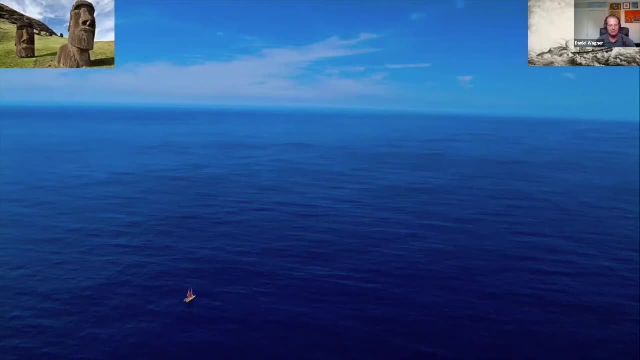 There's many suspected shipwrecks in the area And this again is important for conservation. I mentioned that some of the first marine protected areas were around coral reefs. Likewise, some of the first ones were to protect a cultural resources or shipwrecks. 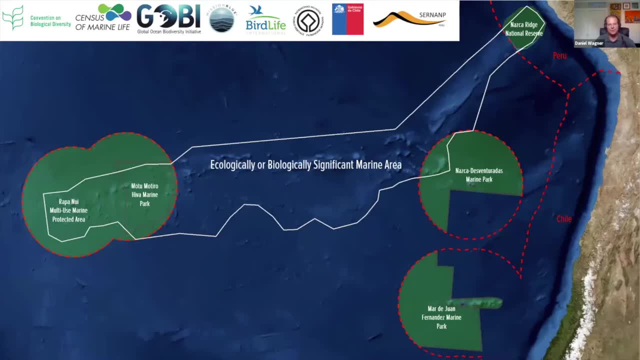 And with that I'll just mention that, because this area is so important for both natural and cultural resources, some of its area has, that is, within the jurisdictions of Peru and Chile, has already been protected, But the biggest part of these ridges, this whole area here in white, is not yet protected. 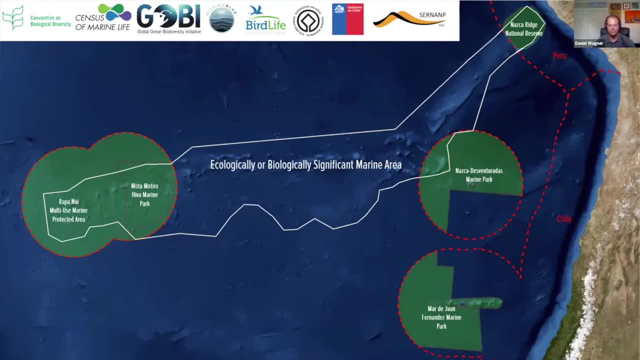 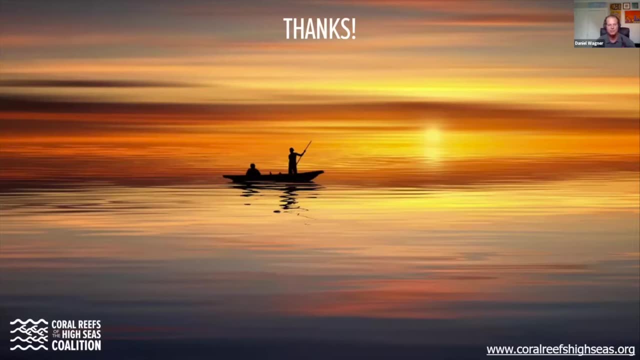 And that could be one of the first priorities moving forward. And with that I'll just finish by mentioning that this is a work by the broader collaboration. many people contribute to that and point you through our website where you can find a lot more information about this work. 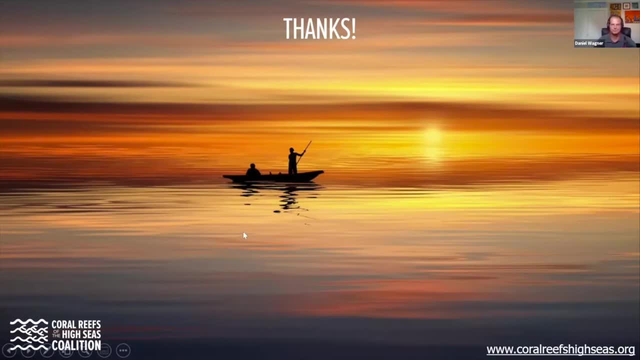 Thanks so much. Thank you, Daniel. This is a wonderful and interesting presentation And I didn't realize until I saw those kind of statues and I realized, oh, that's the East Island. So anyway, my suspicion- but we can discuss this later- is: 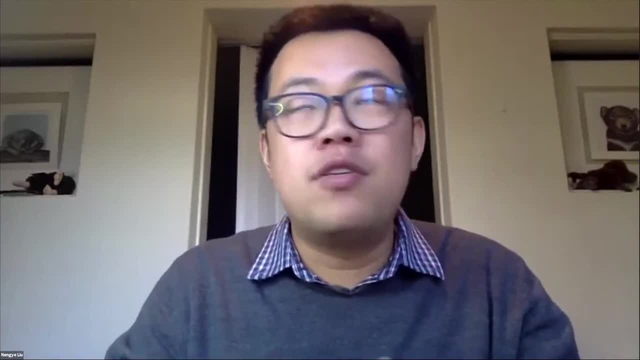 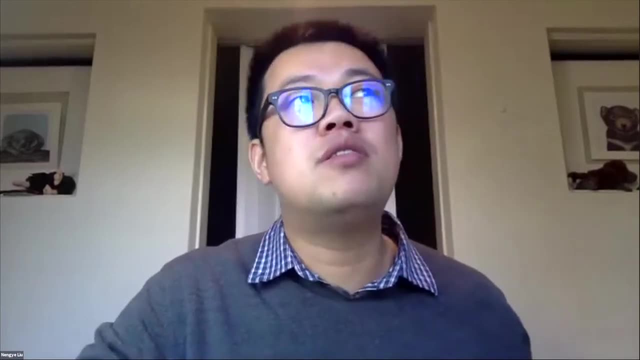 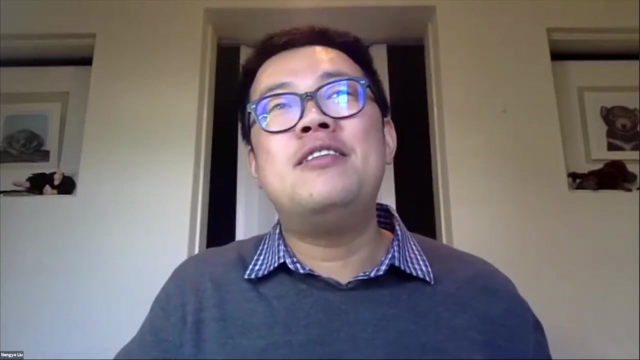 I mean it's not about the importance, of course. I mean that's of course the importance of protecting the coral reefs. But my suspicion is: to what extent could this new BB&J agreement help, Because it seems that people now have a very high expectation. 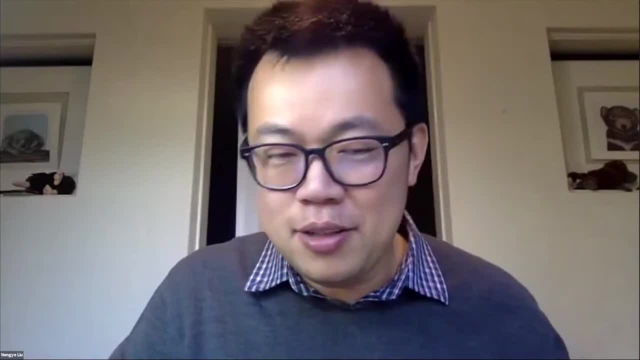 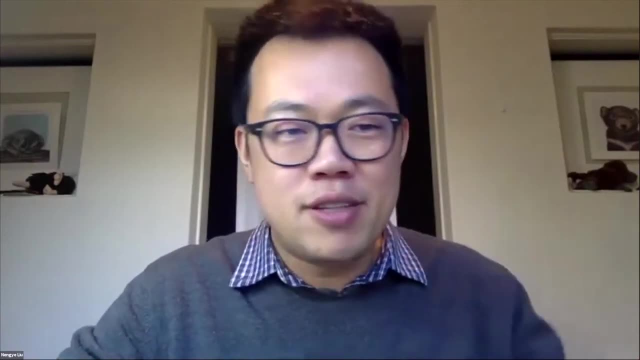 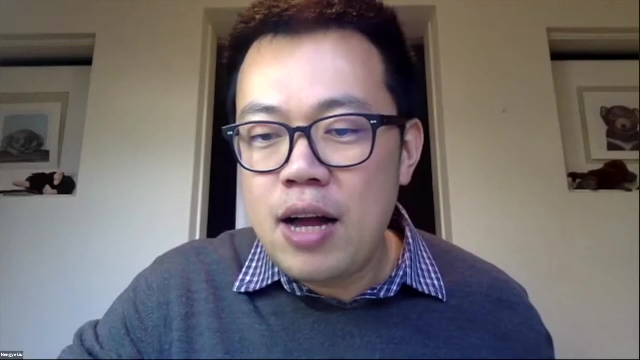 of this new BB&J agreement, but I'm not too sure. So we can further discuss that, But without further delay. our next speaker is Professor Karina Oliveira. All right, Professor Oliveira is a professor at the University of Brazil from School of Law University of Brasilia in Brazil. 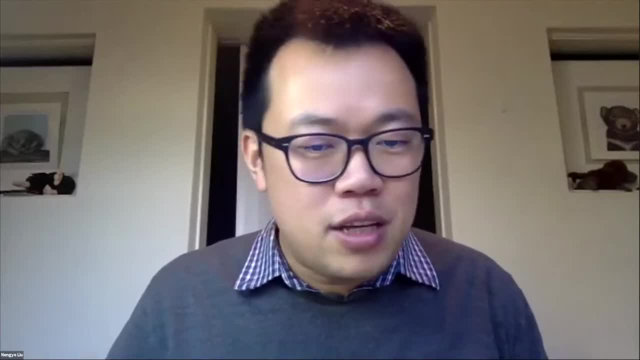 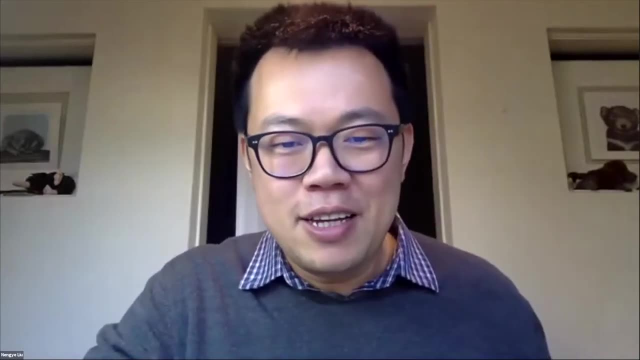 So Karina is going to present us a very interesting- And I think I haven't really thought about this before because now we have lots of discussions on the climate litigation, But what Karina is going to present is the possible contributions of the future BB&J. 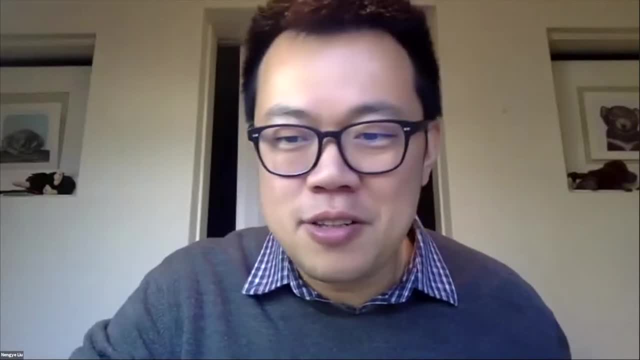 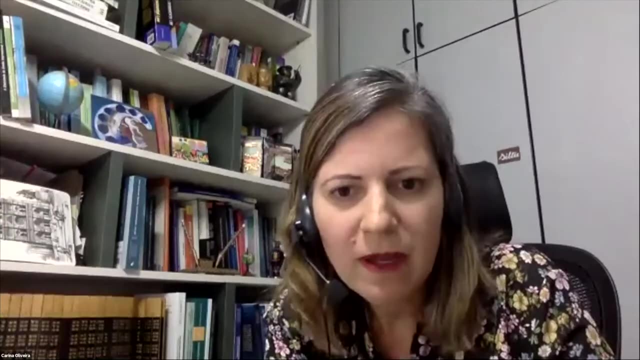 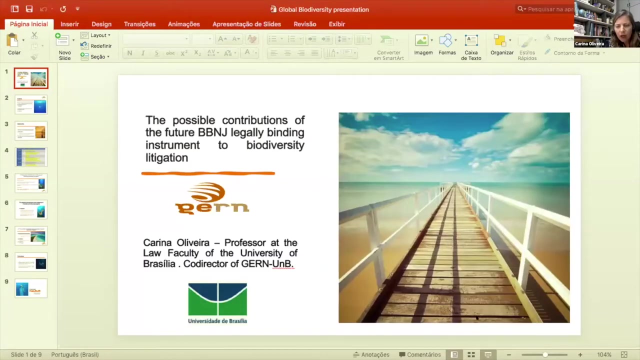 legally binding instrument to biodiversity related litigation. I really look forward to hearing your thoughts, Karina. KARINA OLIVEIRA RODRIGUEZ ARRANNO- So let me just share my screen, OK, Is that OK? OK, great. 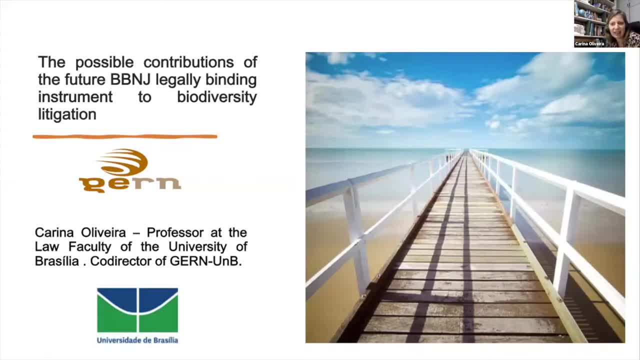 So, thank you, Professor Mingy Liu. I'm really happy to be here with you. Thank you and thank for all the organizations for this opportunity to participate. So my presentation will begin now. try to add one element to the debate, which is in the possible contributions of the future. 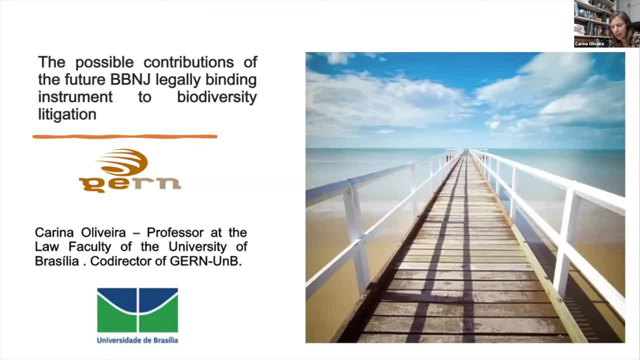 BBNJ legally binding instrument to biodiversity litigation. So for this conference I thought it would be interesting to join the BBNJ future treaty issues, with biodiversity litigation being the first one future treaty, one instrument to strengthen principles, definitions and obligations that could be used in biodiversity.